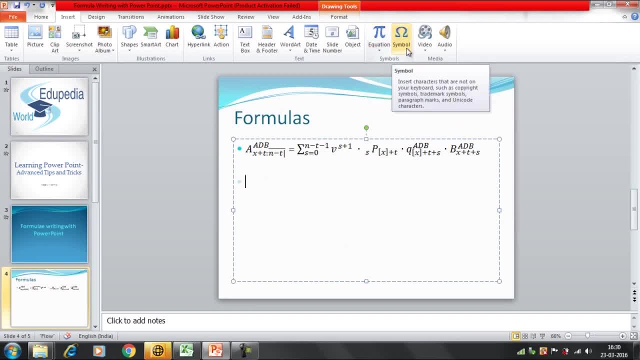 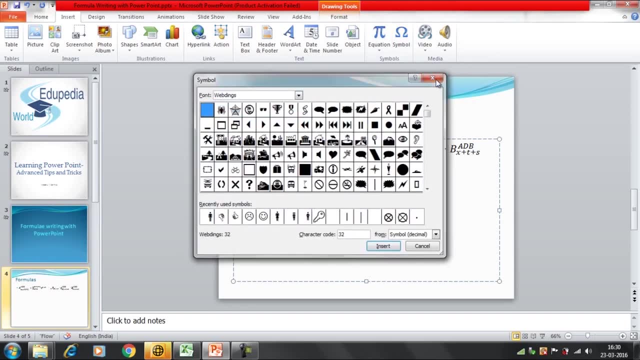 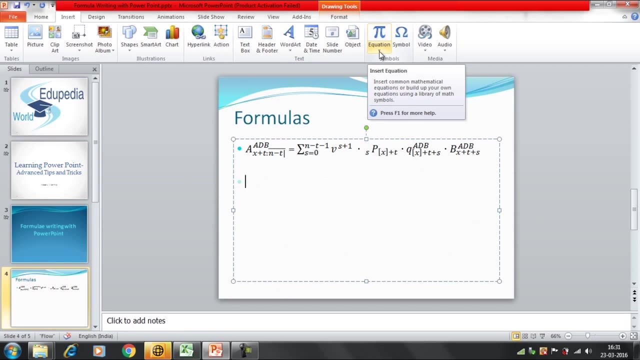 I will click on equation and symbols. If you want to insert a particular symbol, then you can click here and you can search for the symbol and click on insert. Otherwise, if you want to write down the entire equation or the mathematical expression you want to represent in the PowerPoint, then you need to click on equations. 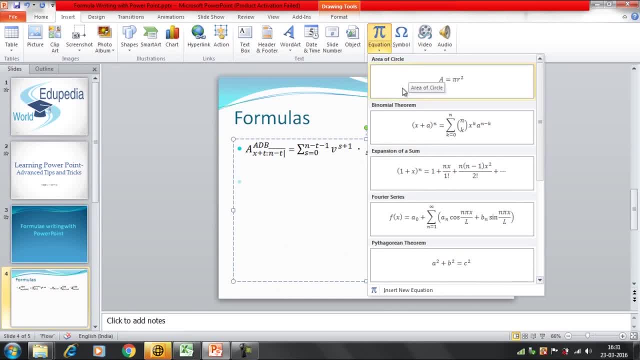 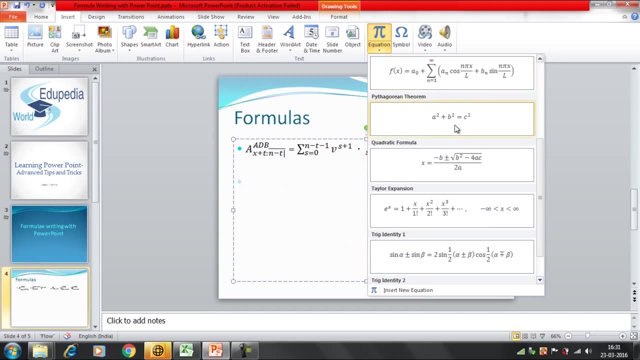 And there are some basic examples here: Expansion of a sum, Fourier series, etc. So you can select the type of series in which you want to represent your data, and you can carry on. For example, if you want to write a Pythagorean theorem, then you can select here. 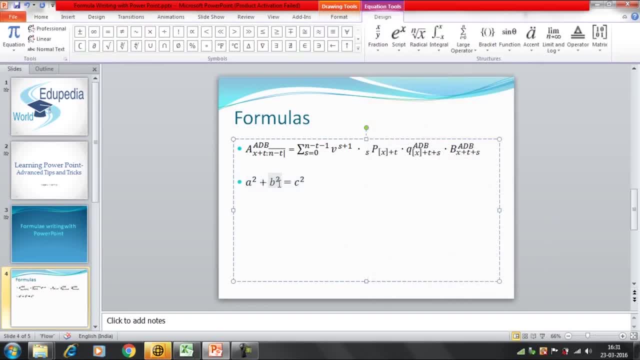 Now, if you want further, you can add here like a square plus b square. Now I want to write here c square, So you can insert here a expression here. This is a script symbol. You can insert a kind of this script. You can write here in this box: c. 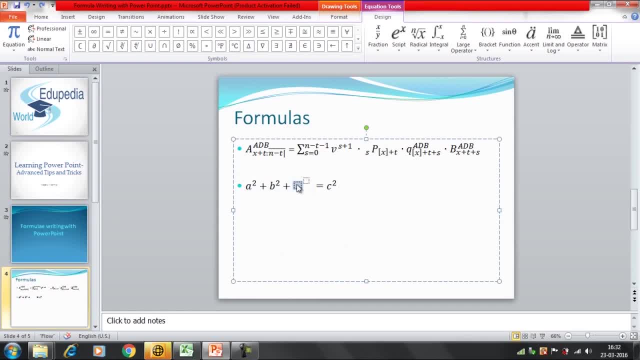 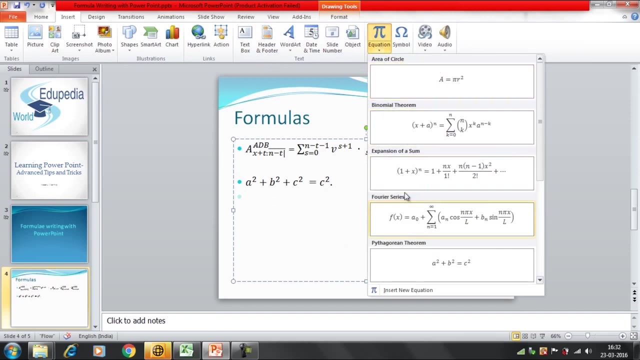 In this way you can insert the equation first and after that you can modify the equation. Now further moving, let's suppose you want to design an entirely new equation which is not a part of the equation system. Then you can suppose you won't find the type of equation that you want to write in this list. 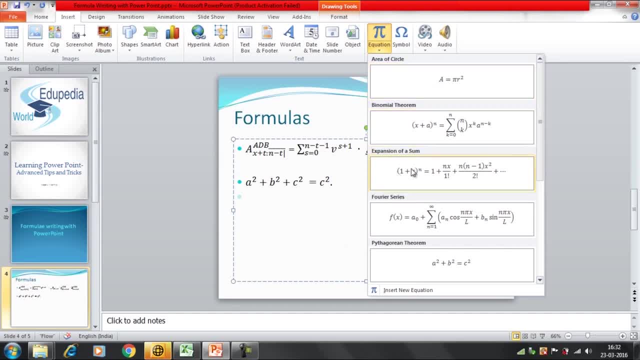 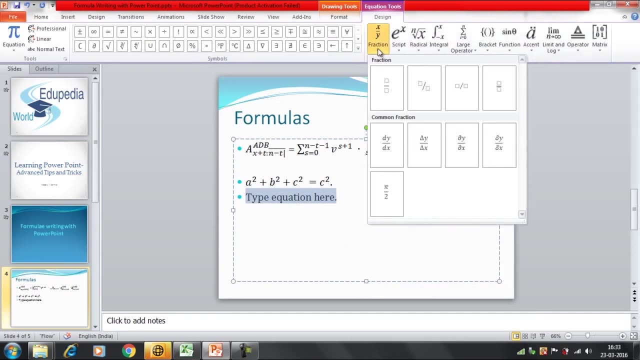 Expansion of a sum Fourier. It's not here. You want to design altogether a new series or a new equation? Then you can click here, insert a new equation, And you have a lot of options available, like fraction. What kind of thing you want to write here? 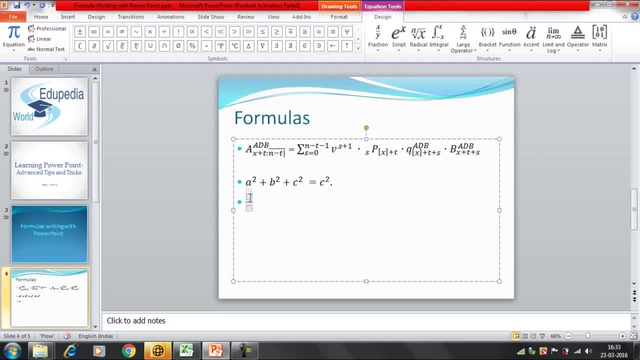 I want to write a fraction here, So I'll write here a and in this box I'll write here b. Even if you want to change here, like you want to represent a square by b square, Then again we'll select this script option.